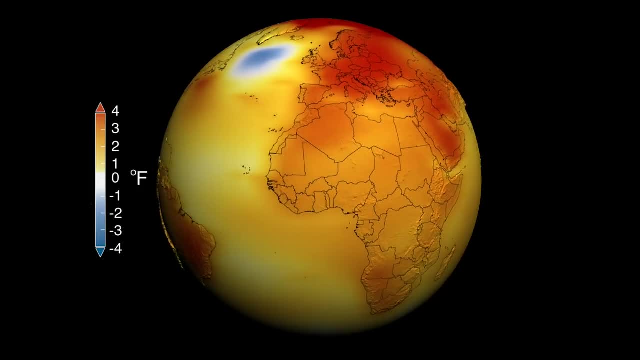 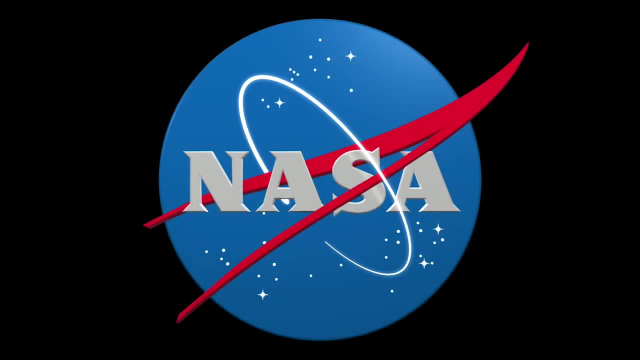 They're working to understand how more and more plants absorb carbon dioxide. NASA studies are: Garcia Kime. When plants Defence, They're working to understand how much carbon dioxide they absorb. They're working to understand how much carbon dioxide they absorb, aware that ground Arctic energy is running more than them. � They're working to understand how much carbon dioxide they absorb YTän Rn 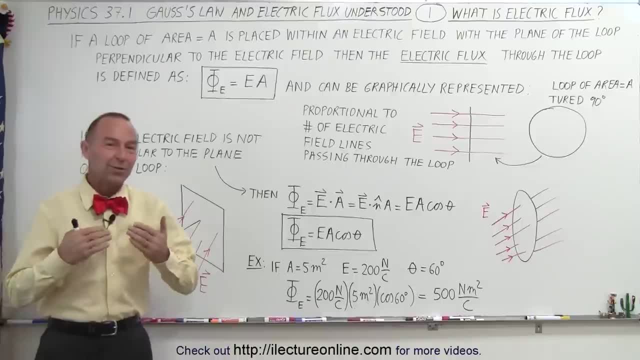 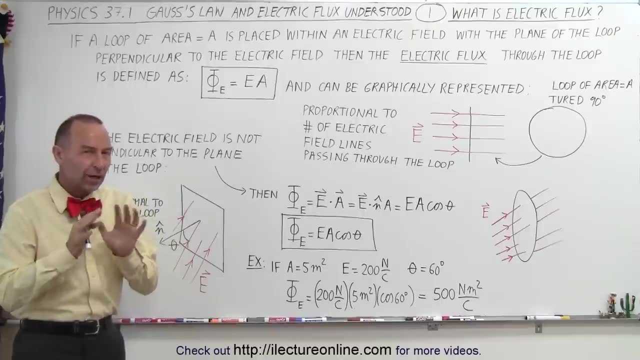 Welcome to our lectern line. Here we're starting a new set of videos on Gauss's law and the electric flux to get us a better understanding. So we're going to talk a little bit more about the details of all that, But we're starting with the concept. what is electric flux? and actually it's kind of 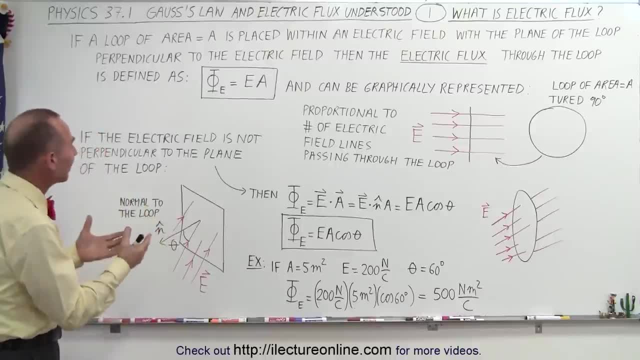 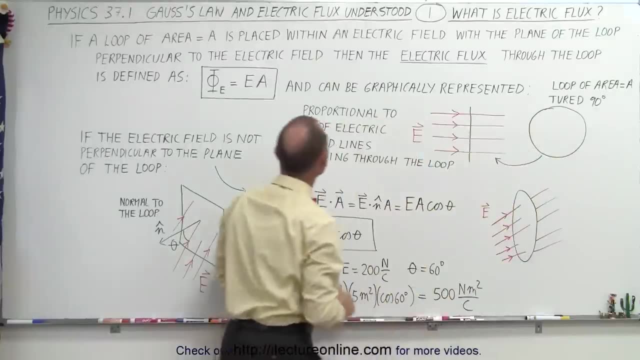 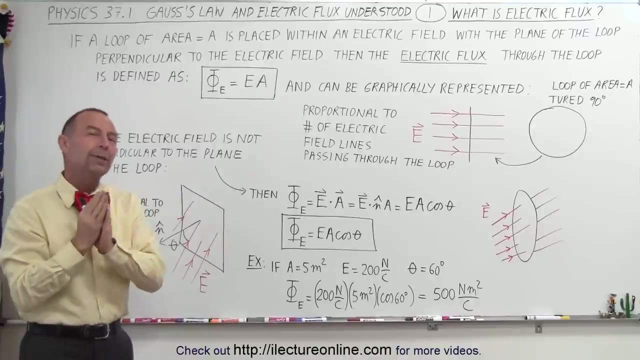 difficult to imagine what it is. So the best way to define it is as follows: Let's say that we have a loop of area A, just a simple loop like this, and the area of that is A, And we place that loop within an electric field such that the plane of the loop is perpendicular to the field. So here's. 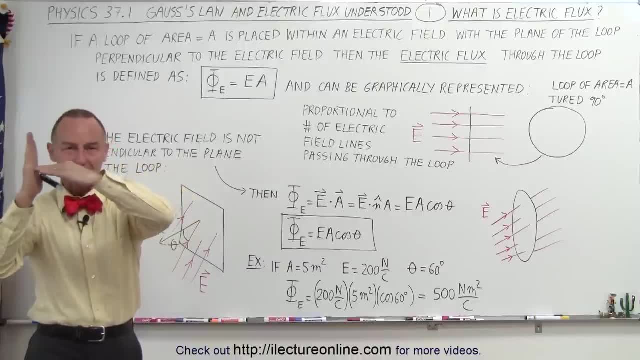 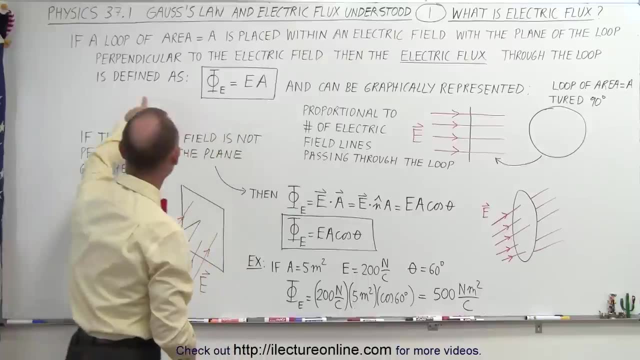 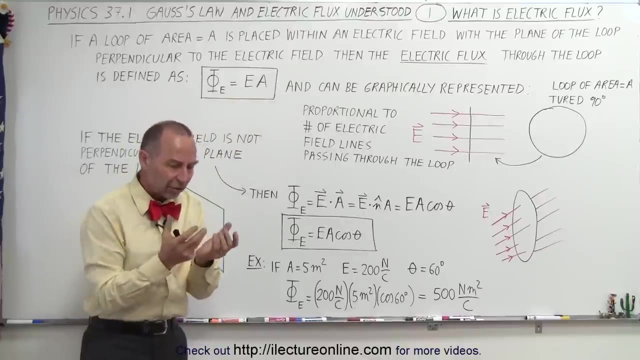 the loop. here's the field. the electric field is perpendicular to the plane of the loop. Then we can say that the electric flux through the loop is defined as the product of the magnitude of the electric field in the area of the loop. So it's actually the product of two things. You multiply the strength or the magnitude of the. 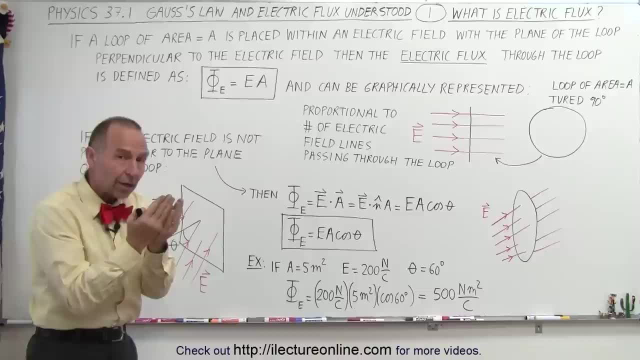 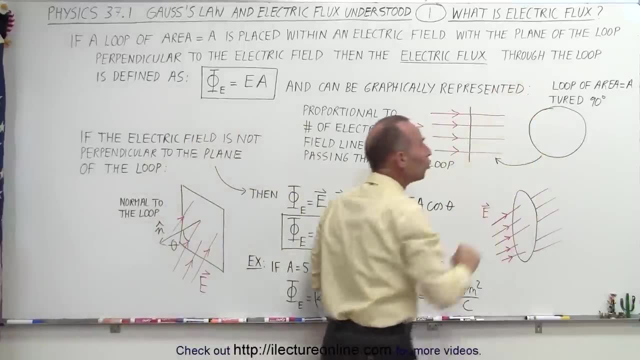 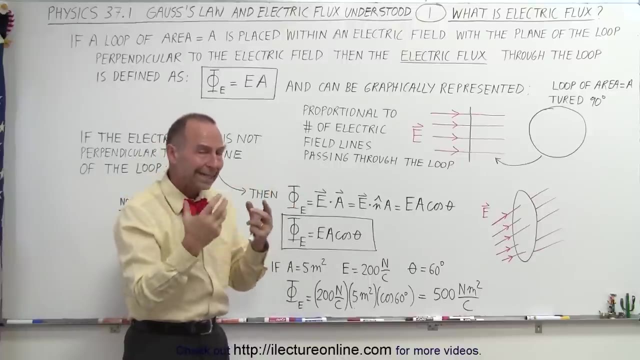 electric field times the area of the loop. That product is the flux through the loop. So the important thing also is that we talk about flux through a loop. Flux by itself doesn't really mean much, but if we go through a loop like a conductor or wire then there's a lot of meaning. 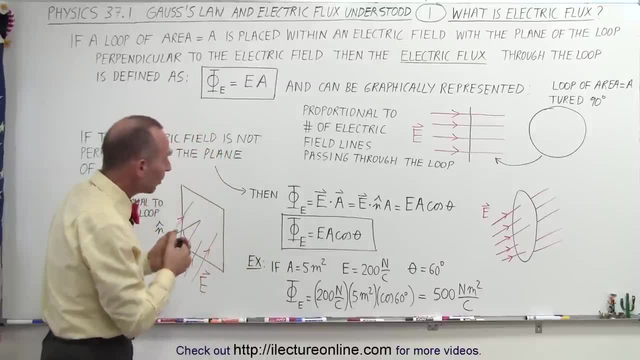 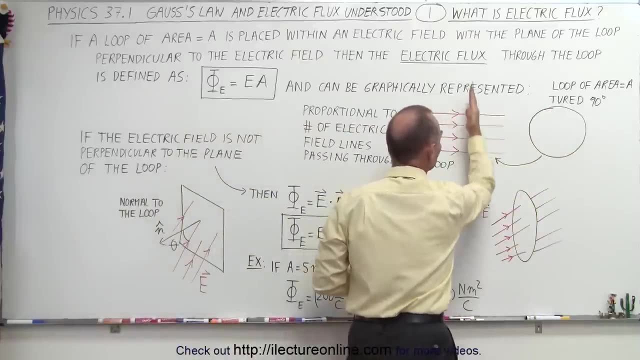 to it. That's the concept of flux. So we can graphically represent it as follows: So let's say that we take the loop here and we turn it 90 degrees. So now we're looking at the loop edge on and now we have an electric field present And we can draw electric field by drawing the electric 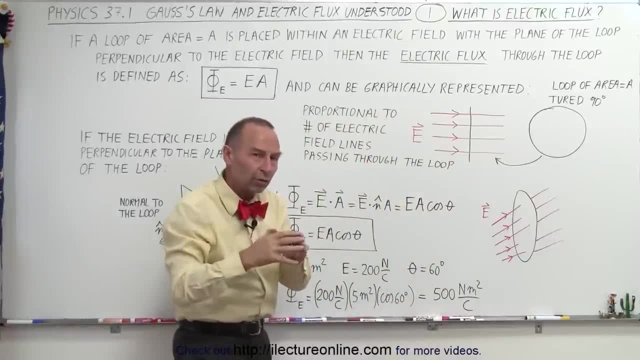 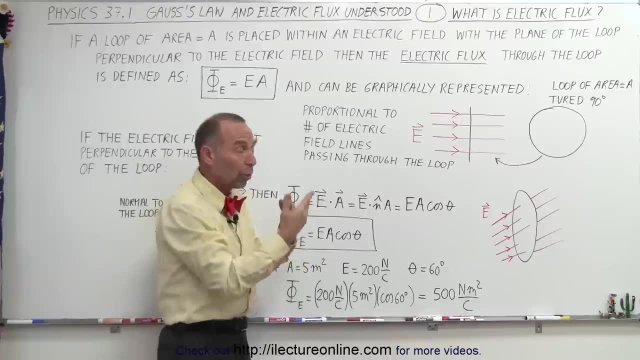 field lines and those are kind of synonymous to the flux, or at least proportional to the flux. The stronger the field, the more lines that we draw. So you can kind of graphically imagine: the more lines you see, the greater amount of flux that you have through the loop.